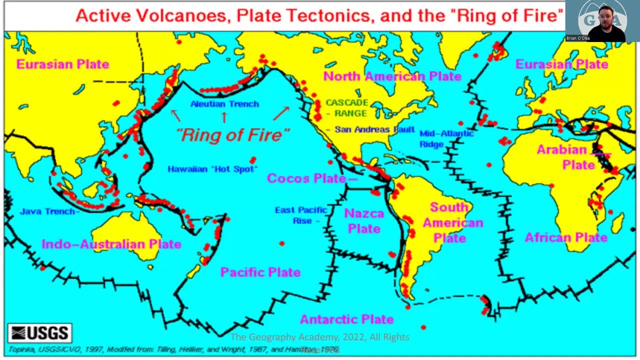 very thin indeed. So we're living on this thin crust and we can see some of it forms continents and then some of it is in the ocean, And we can also see the red dots that are around of active volcanoes. So this is showing us, then, that a lot of 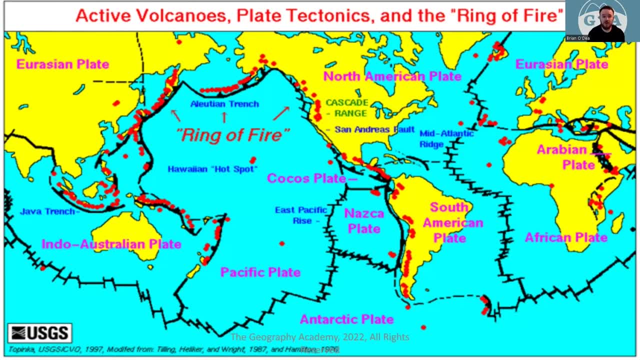 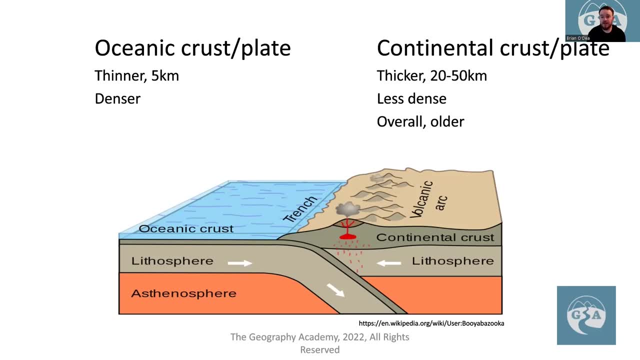 volcanoes do have a correlation with tectonic plate boundaries. We've got two types of crust that we talk about. We've got the oceanic and the continental. The oceanic is thinner, the continental is thicker. However, the oceanic, while it's thinner, is denser. And then the 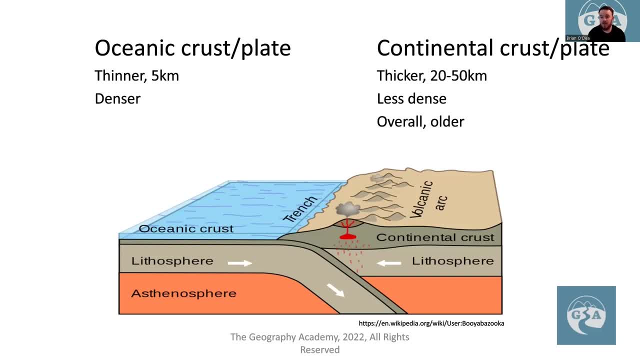 continental overall is going to be less dense, even though it's thicker. So if you're having trouble kind of thinking about what does that mean? Think about if you had an inflatable bed on a swimming pool, right, And you can lie on it, right. The idea is that there's a lot of mass. 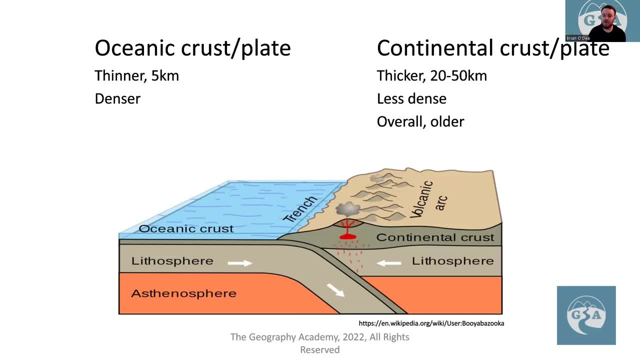 but the density is still much lower than the water, right, Because there's air there that is less dense, So that keeps you afloat, Whereas if you were sitting on the bed and then suddenly you dropped your phone into the pool, what you'd find is the phone would sink down to the very 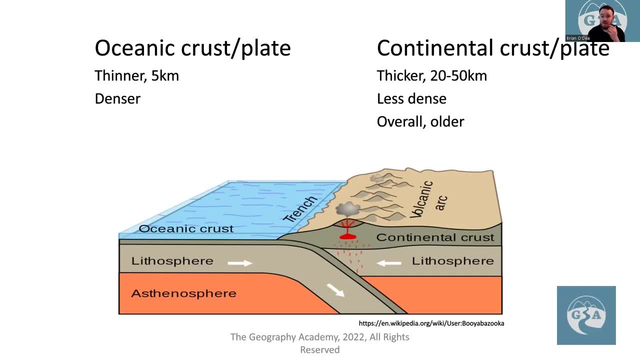 bottom right. Even though it's much smaller, it's denser, So it's going to sit lower, And that way the oceanic crust, while it's smaller, is going to sit lower on the asthenosphere and the continental crust is going to be less dense and it's going to sit slightly higher on the. 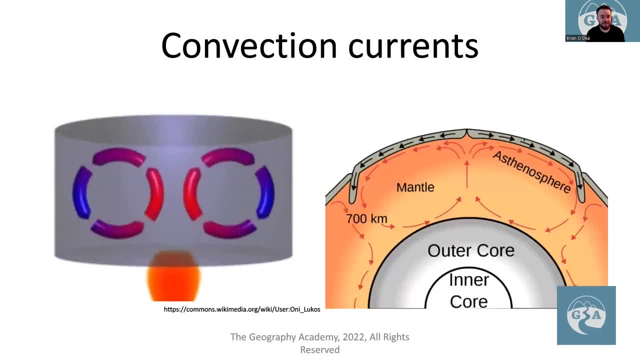 asthenosphere, even though it's bigger, All right. So another process we have to think about are convection currents. So what's going on is the heat from the mantle is causing the magma to rise inside, And as it reaches the top, it's then going to cause the convection current to 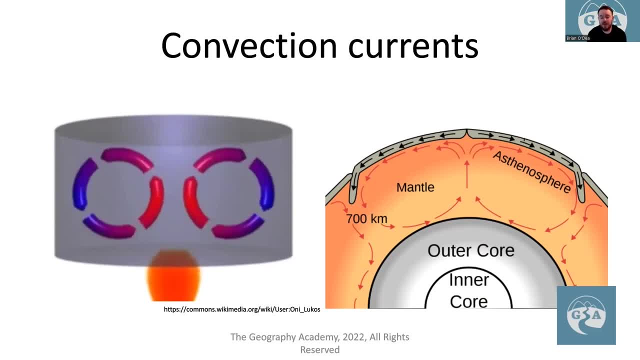 move either side, And this is going to make it move in the direction of the convection currents. The magma then, as it's moving, is going to become more dense because it cools down- Again we're talking about density- And this is going to cause it to return to the core, where it will 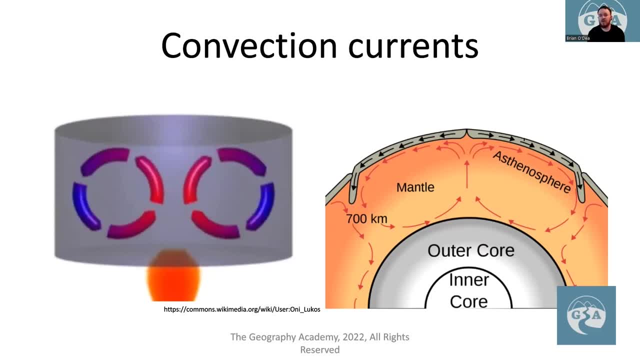 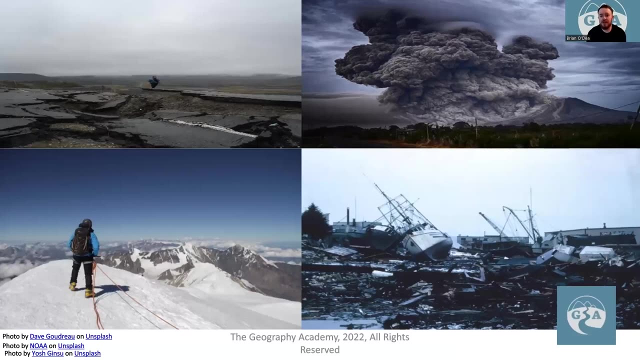 heat up and go around again. So when you're starting off really any question about tectonic plates, we would probably say things like, yeah, convection currents are kind of beginning of the explanation, the first process to go through, All right. So what are the results of these tectonic plate movements? Well, as always,